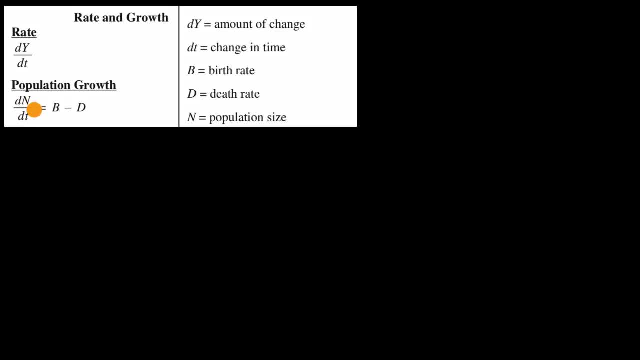 in a biology class, But what we'll see in this video is that this formula is actually just trying to express something that's fairly intuitive and something that you actually don't even need calculus or even much algebra. but then we'll connect it to this. 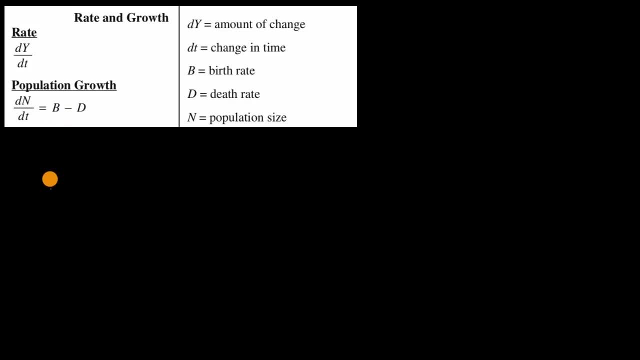 to see that it all makes sense. So, putting this aside, let me just ask you a simple question. Let's say we're studying a population and we see that the birth rate, the birth rate of this population, is equal to 60,. 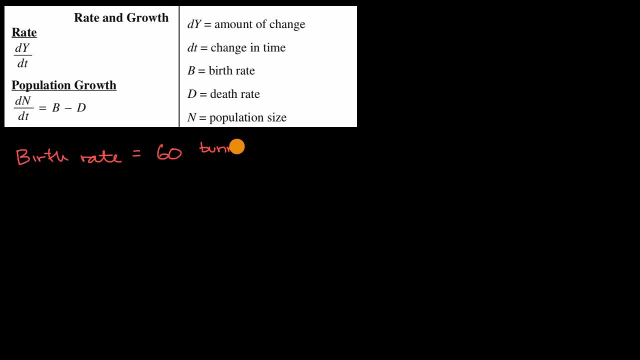 let's say we're studying a population of bunnies- 60 bunnies bunnies per year- And let's say we know that the death rate of bunnies death rate is equal to 15 bunnies bunnies per year. 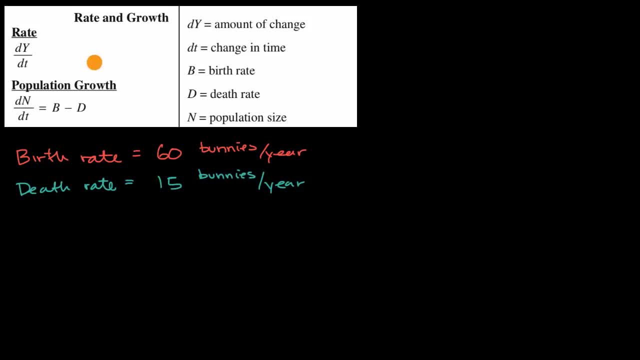 Now, without even paying attention to this formula sheet up there, what do you think, given this data, is the population, population growth rate for this population of bunnies? Pause this video and see if you can answer that Well, your population growth rate. if you think about. 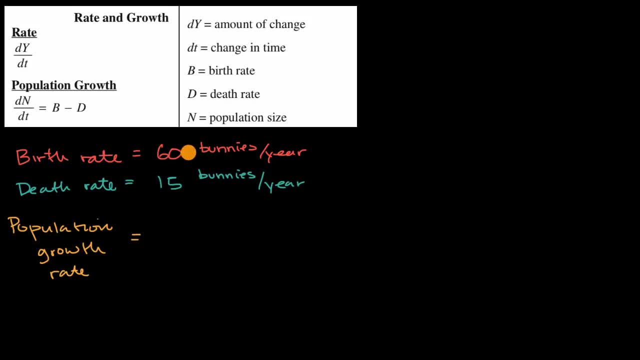 just even say a given year. in that year you'll grow your population by 60 bunnies per year. so you will grow 60 bunnies per year. So you would grow by 60 bunnies per year, but then you would shrink by the 15 that died. 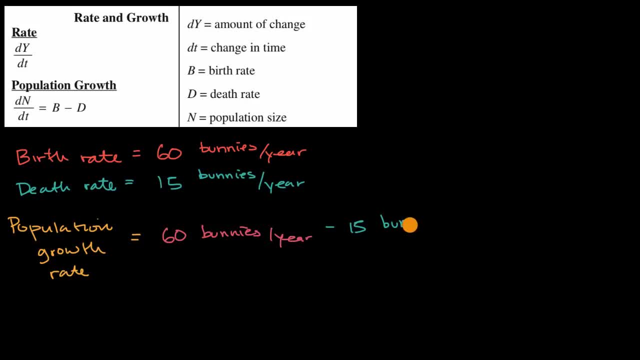 So it would shrink by 15 bunnies, bunnies per year. And so in that year you would net out 45 bunnies. And that's a rate because you're saying per year. So you would grow by 45 bunnies, bunnies in that year. 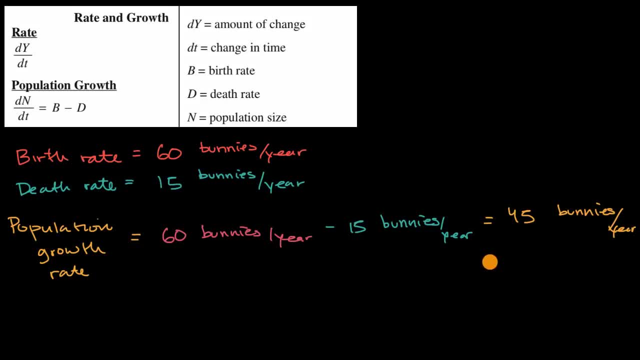 And that would be your population growth rate. Now, the thing that we just talked about, we just did very intuitively. you don't need advanced math to think through what we just did. That's exactly what this formula is saying, This notation where you say d, something, dt. 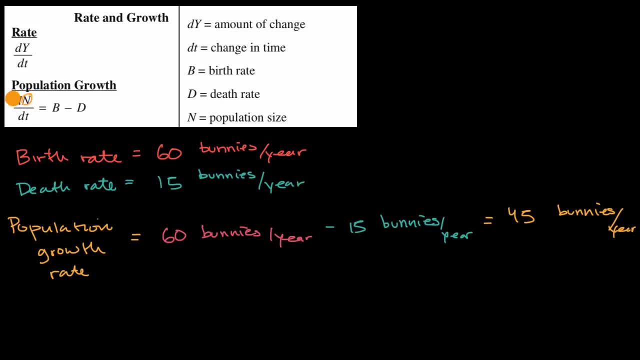 this is the rate at which this something is changing with respect to time. So this is just a fancy way of saying what is the rate at which our population is changing with respect to time. There's other ways that you could have written that.